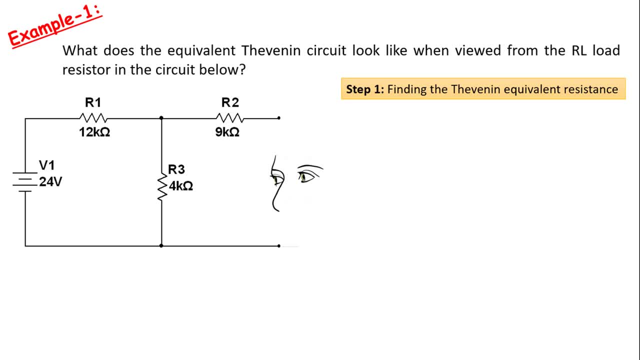 Now we can look at the circuit circuit between these two points. Then we need to open-circuit the current sources and short-circuit the voltage sources. Since there is only one voltage source of 24 volts, we must short-circuit it. Now we can find the Thevenin equivalent resistance. 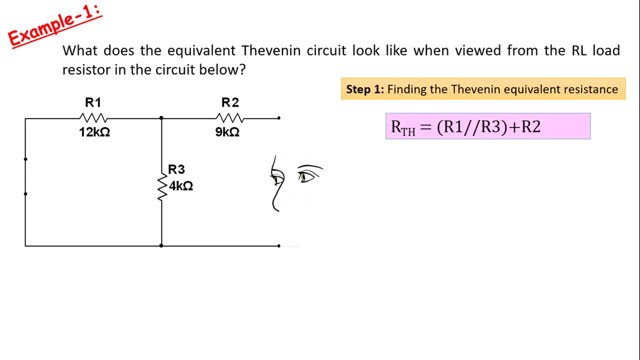 Here resistors R1 and R3 are in parallel. R2 is connected in series with them. We can write this mathematically as in this formula: 12 kilo-ohms and 4 kilo-ohms are parallel to each. 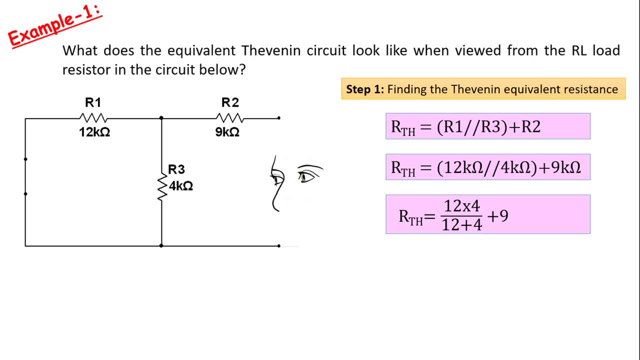 other and 9 kilo-ohms is in series. Since 12 kilo-ohms and 4 kilo-ohms are in parallel, the equivalent will be 3 kilo-ohms If we add this value with the series 9 kilo-ohms. 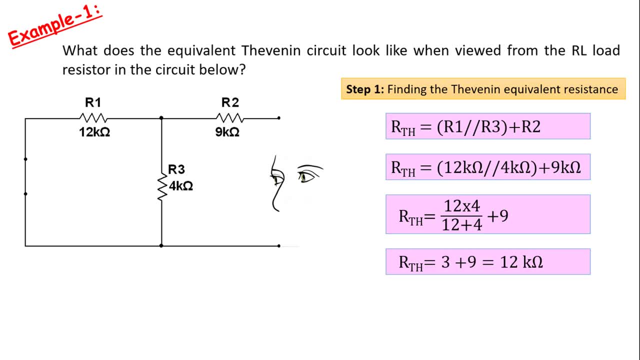 we find the Thevenin equivalent resistance as 12 kilo-ohms. Step 2 is to find the Thevenin open-circuit voltage. If we find the voltage here, by making an open circuit where the RL resistor is, we can find the Thevenin open-circuit voltage. 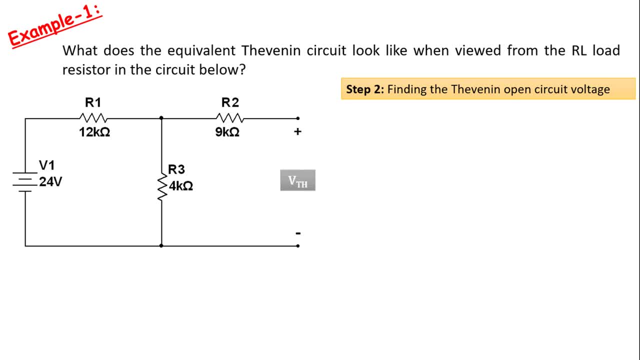 The voltage here is actually the voltage across the 4 kilo-ohm resistor R3.. Because the load resistor is open circuit, no current flows through the 9 kilo-ohm resistor R2.. Therefore this resistor has no effect on the circuit. To find this voltage, if we divide the source voltage, 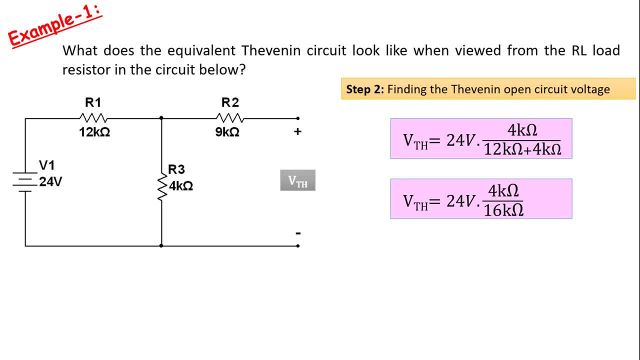 of 24 volts, proportional to the resistor values, we can find the voltage falling on the 4 kilo-ohm resistor. We can write this mathematically as in this formula: For this we find the Thevenin voltage as 6 volts. 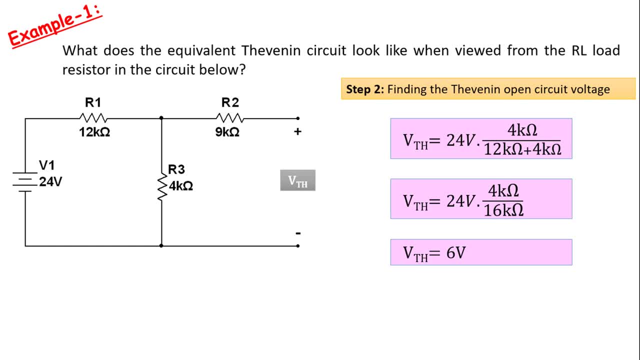 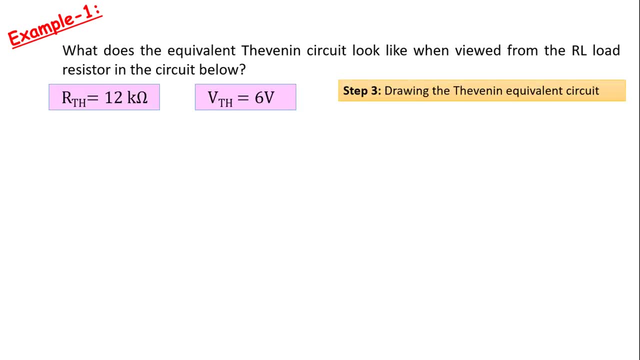 We found Thevenin's equivalent resistance and Thevenin's open-circuit voltage. The third and last step is to draw the equivalent circuit of Thevenin. The Thevenin voltage is shown as an independent voltage source. The equivalent resistance of Thevenin must be connected in series with it. We can also connect: 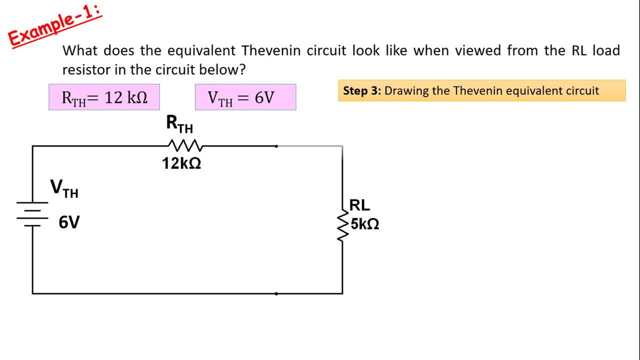 the load resistor RL to this circuit. From now on you can also find the load, current or voltage RL if you want. This is the Thevenin equivalent circuit of the circuit in this example. according to the RL load resistor. friends, If we do the source conversion here, that is, if we show this: 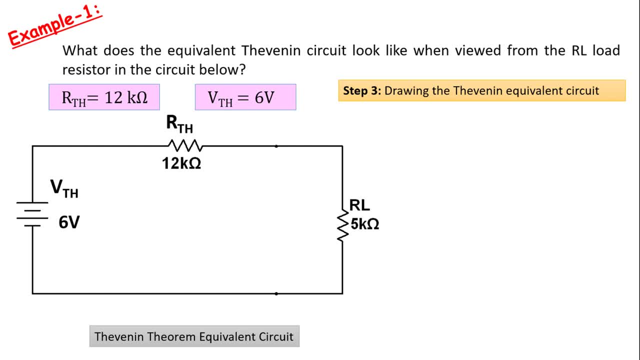 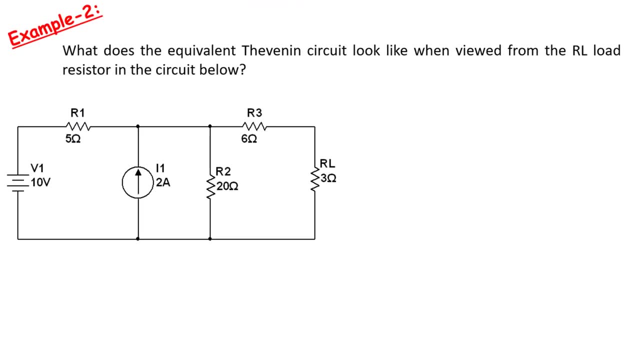 circuit as a current source, we get the Norton equivalent circuit. Let's do one more example for better understanding. Again, in this example let's try to find out what the Thevenin equivalent circuit looks like when viewed from the RL load resistor. 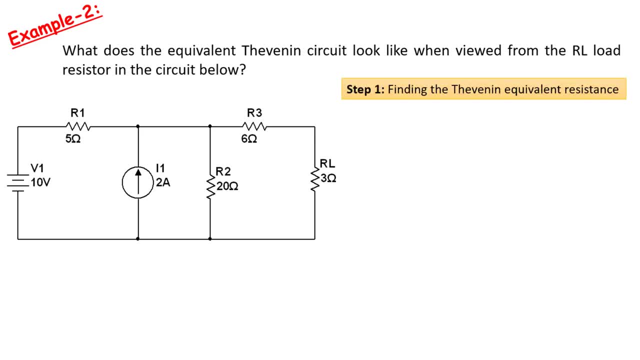 Again, the first step is to find the Thevenin equivalent resistance. For this we first need to remove the RL load resistor from the circuit, where we will look at the circuit. Now we can look at the circuit between these two points. Then we need to open. 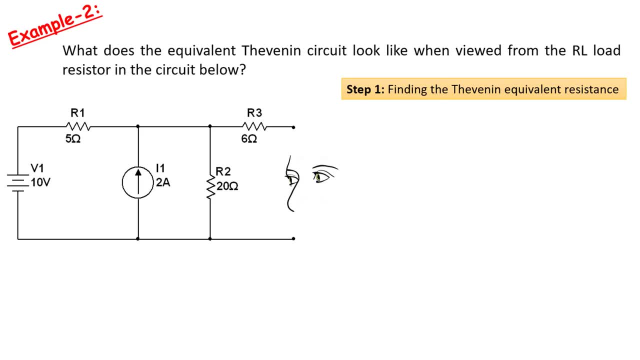 circuit the current sources and short circuit the voltage sources. Here we need to short circuit the voltage source of 10 volts and open circuit the current source of 2 amps. Now we can find the Thevenin equivalent resistance. Here resistors R1 and R2 are in parallel. Resistance R3 is 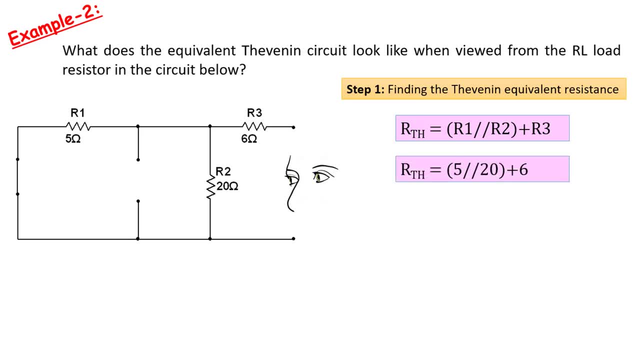 connected in series with them. We can write this mathematically as in this formula: 5 and 20 ohms are parallel to each other and 6 ohms is in series. Since 5 and 20 ohms are parallel, the 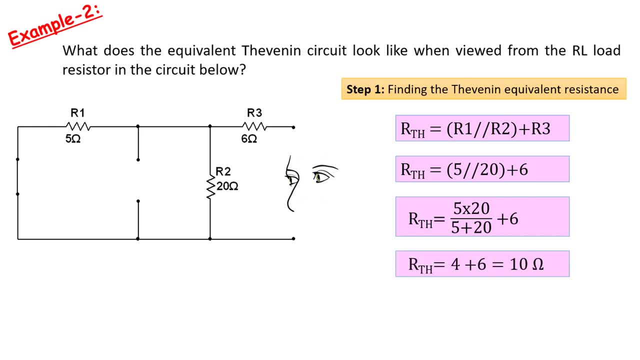 equivalent will be 4 ohms. If we add this with 6 ohms in series, we find the Thevenin equivalent resistance as 3 ohms per current. And if we add 40 mu to each number, the equivalent willalleré's must have. 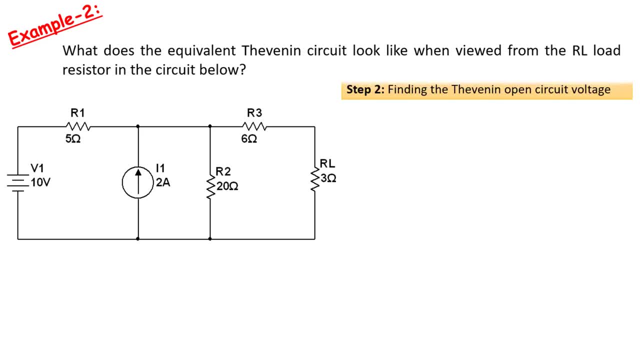 10 ohms. Step 2 is to find the open circuit voltage of Thevenin. If we find the voltage here, by making an open circuit where the RL resistor is, we can find Thevenin's open circuit voltage. The voltage here is actually the voltage across the 20 ohm resistor R2.. 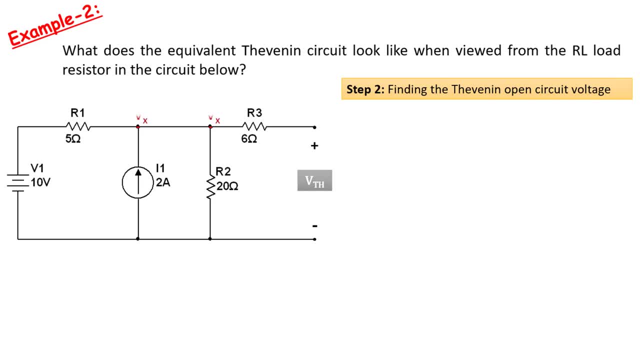 To find this voltage it is enough to find the voltage at the point I indicated as Vx. since the place where the 6 ohm resistor R3 is located will be an open circuit, this resistor has no effect on the circuit. If we write Kirchhoff's current law at the point Vx according to the node voltages method, 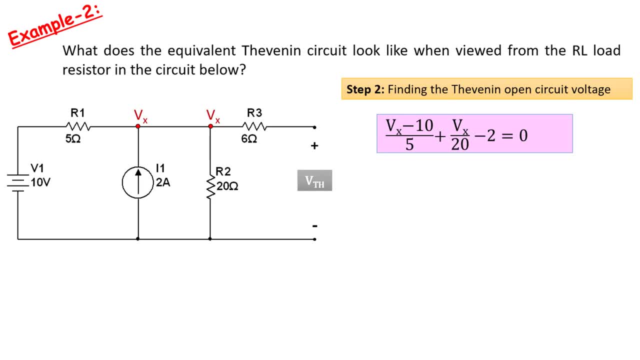 equation: Vx-10 over 5 plus Vx over 20 minus 2, equals 0, will appear. When we simplify this equation, it becomes 5Vx over 20, equals 4.. From here the value of Vx will be equal to Vx over 20 plus Vx over 20, plus Vx over 20.